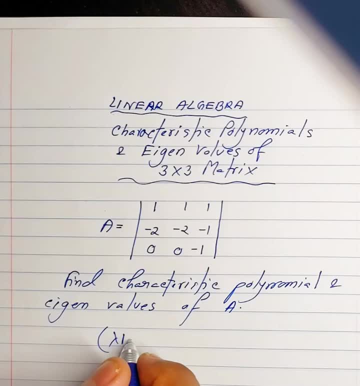 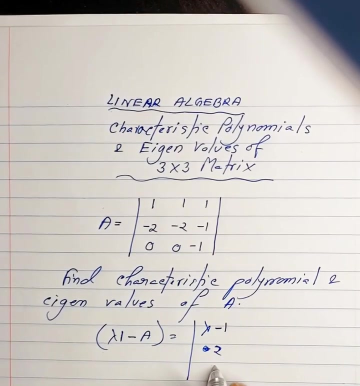 know that characteristic polynomial is lambda identity matrix minus A, which means you take the lambda minus 1 from each of the diagonal matrix. you have minus. you have 2 minus 2. actually your sign will be changed so this will be 2 and it would be 0. then you have. 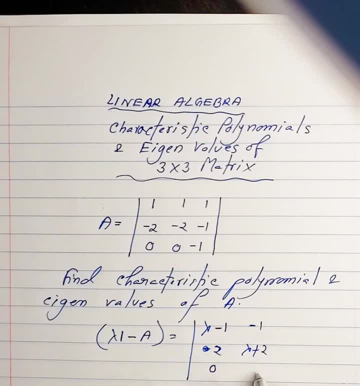 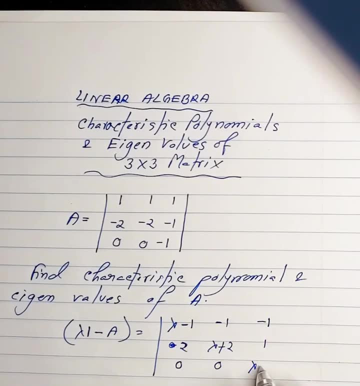 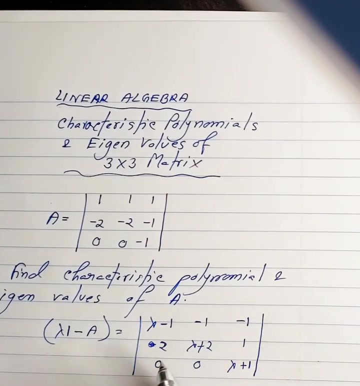 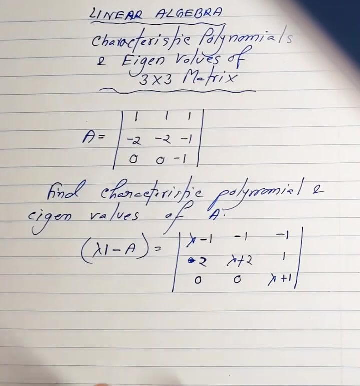 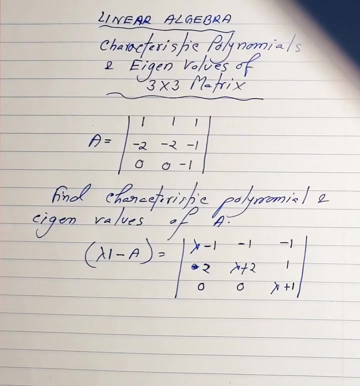 minus 1, lambda plus 2, 0 minus 1, 1 and then lambda plus 1. right Now, this is a matrix that is called a linear matrix. it is astrong characteristics, polynomial, And this is a linear matrix and you can try this method manually. It means it is a linear matrix. 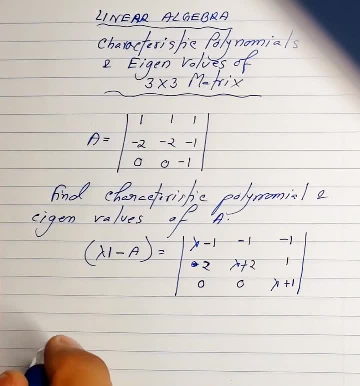 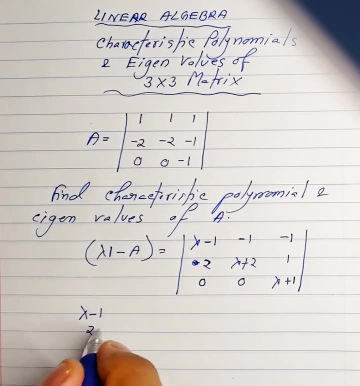 which can be calculated. but then we still need to find partner 1999 when, again, if you know that you have this matrix, which is lambda 1, 2 and 0, and you have minus 1 lambda 2 under plus 2 and 0, and you have minus 1, 1 lambda plus 1, right, so take this 2 against, because you need to take the. 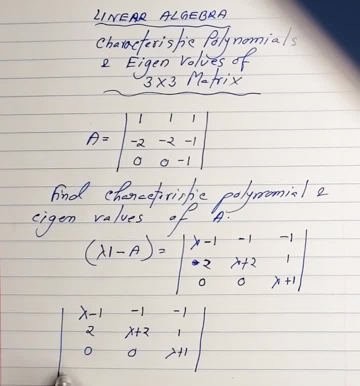 3, 3, metric. so if I go, if I multiply this way, I need to connect three of them, so I can take this again: lambda minus 1, 2 and 0 and the second column again and 0. ok, now what, what should I do now, like? 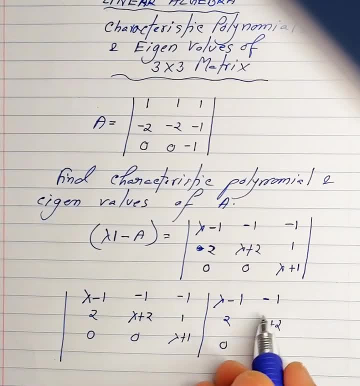 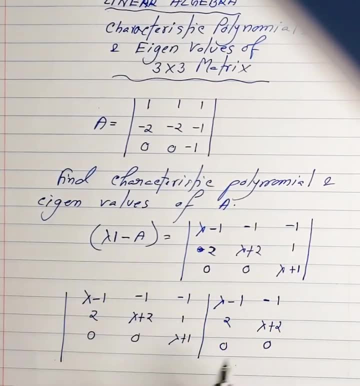 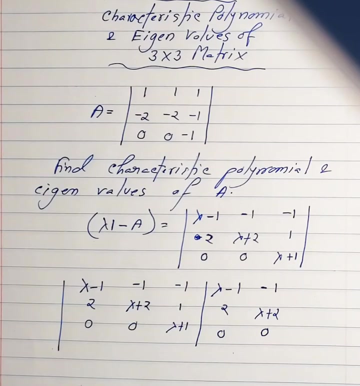 why you're doing it, so that I can just connect them now. multiply this way- ok, first, and then that way. so what you do, like you need this, is the 3- 3 matrix, so three of them should be connected. so I can use a pencil here to show you what I'm trying. 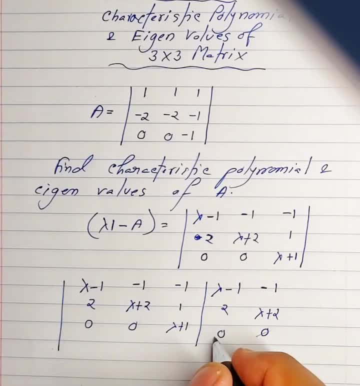 to do so because this is a 1, it's not connected I- these three are the first connected, so I have to multiply these three of them, which gives me minus 2 lambda plus 1 right, and then I have this 3, which is my few multiplies you're. 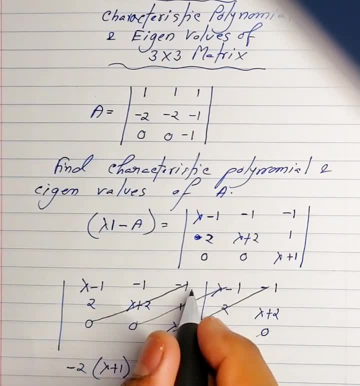 getting 0, and I have this 3, if you multiply you're getting 0, so this- there is nothing else I can take here. but if there is another number, then you have to. just take a suppose you have plot 1 here, so you have one time you want and these, so you have plus lambda. 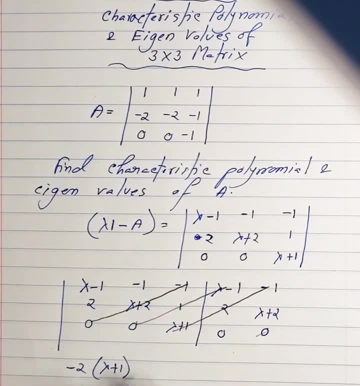 minus 1 again. so you take that. but if you have 0, that's me, I'm not taking anything, because this multiplication is 0 now, that's this part is done. now what to do it without none? the other way, for example, like now, we need to multiply. 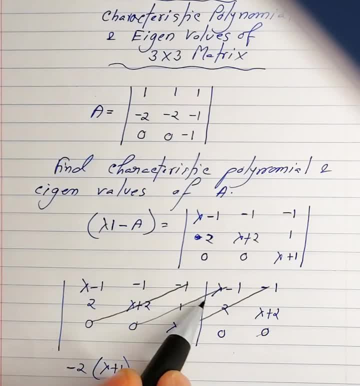 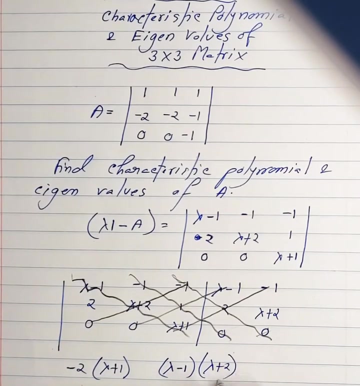 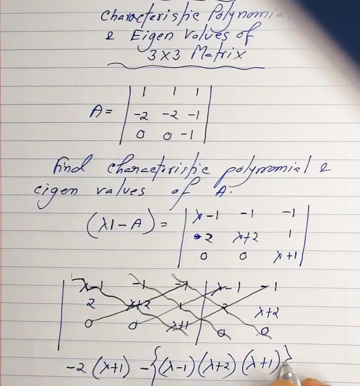 this way. so your first multiplication is lambda- this tree which is 0, then this tree, which is also 0, and now you have this tree which gives you lambda minus 1, lambda plus 2 and lambda plus 1, but the sign in between of them should be negative. so this is the second part of 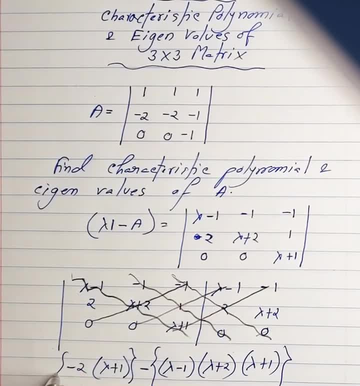 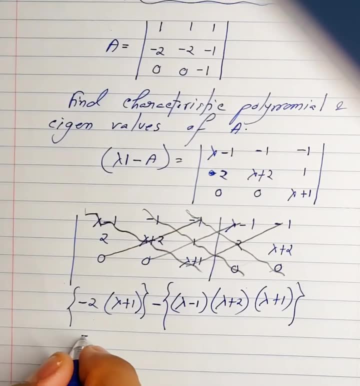 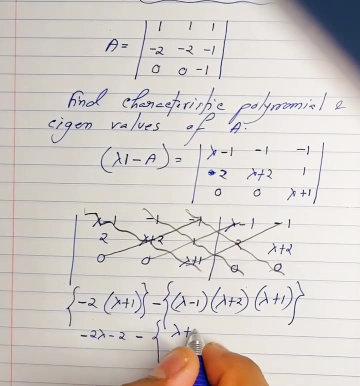 your multiple product and this is the first part of your product. now, all you need to do, you just simplify it. so, from from the first one, I have minus 2, lambda and minus 2, and that gives this gives me lambda 2 and lambda square minus 1. 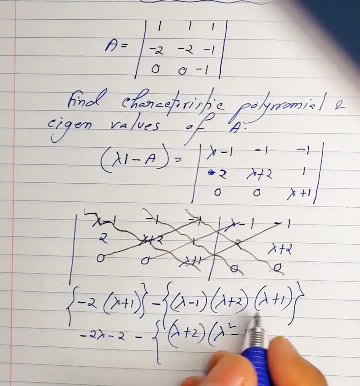 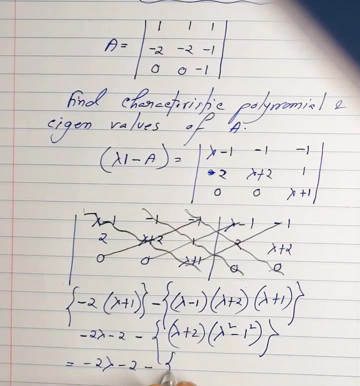 square like a minus B, and a plus B gives you a squared minus B squared. so now we have minus 2, lambda minus 2, and if you just remove the bracket you're getting like if you multiply you get in a lambda cube plus 2, lambda squared minus, lambda minus 2. if